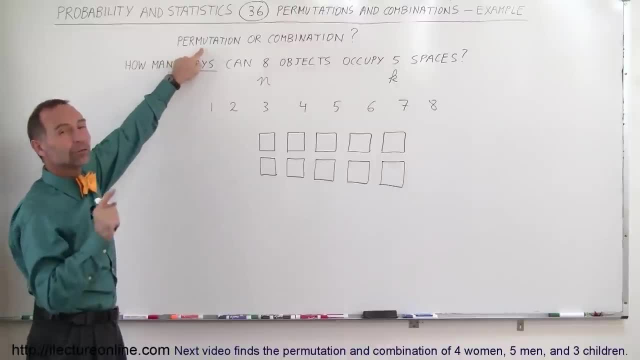 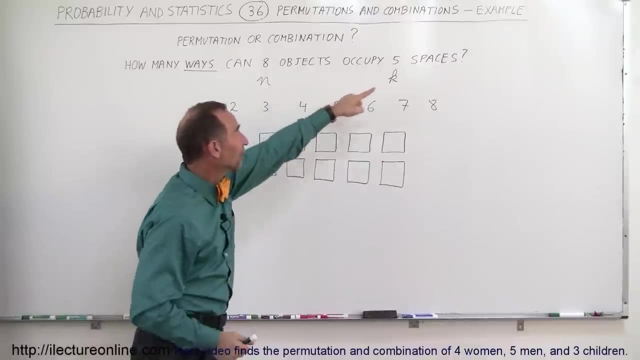 how many ways. that means they usually look for permutations. we're looking for the number of permutations, which means we have eight objects. let's say we have eight numbers: one, two, eight, and then we have five spaces: one, two, three, four, five. So to see what the difference is. 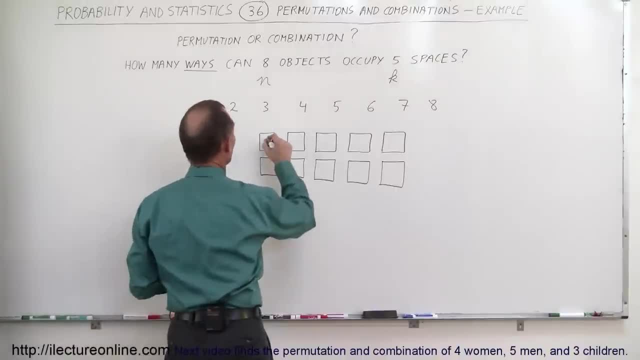 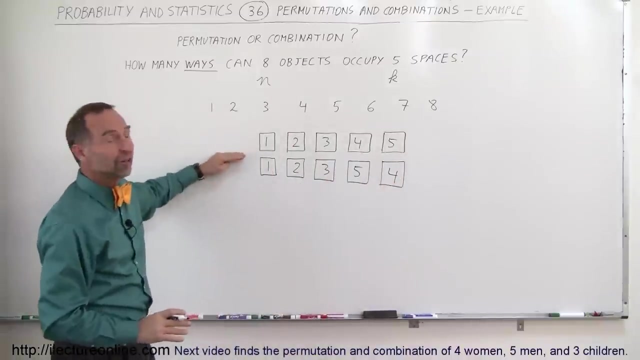 between permutations and combinations. let me put down the first five numbers: one, two, three, four, five. Now if I then write it down like this: one, two, five, three, five, four, when it comes to combinations, there's no difference here. This is one and the. 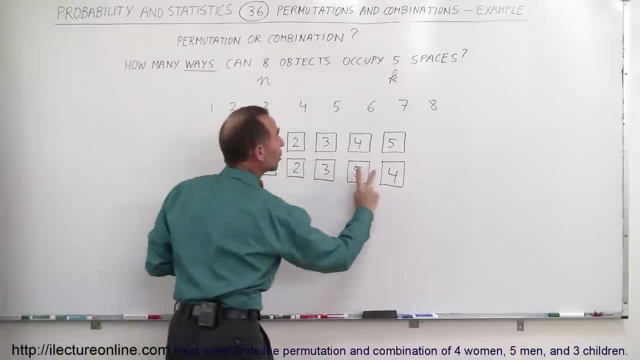 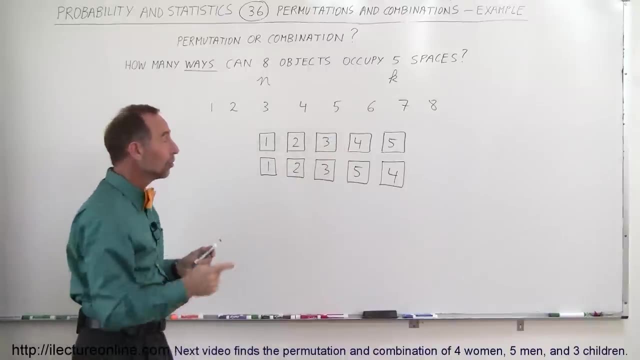 same, but when it comes to permutations there is a difference, because we interchange the four and the five For combinations. you say, well, we have numbers one through five and it doesn't matter how you arrange them, it's all the same thing. So you can imagine when you start shuffling things. 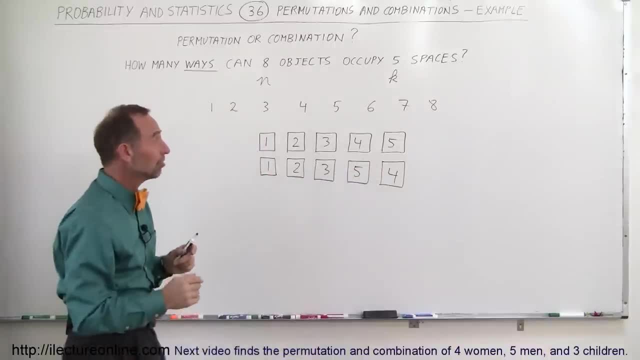 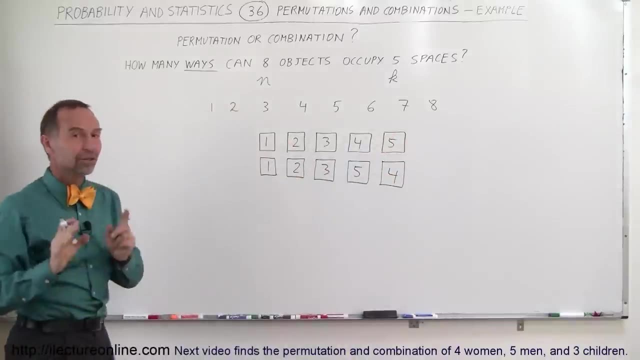 around with the same five numbers. you come up with a lot of different permutations and then you replace the five with a six and then do it all over again. so the number will be very high when it comes to permutations, not so high for combinations. Remember the equation for: 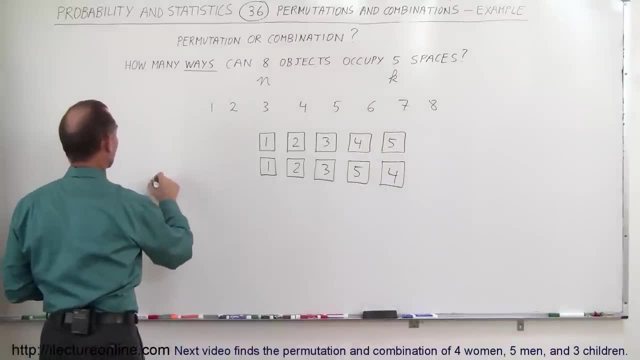 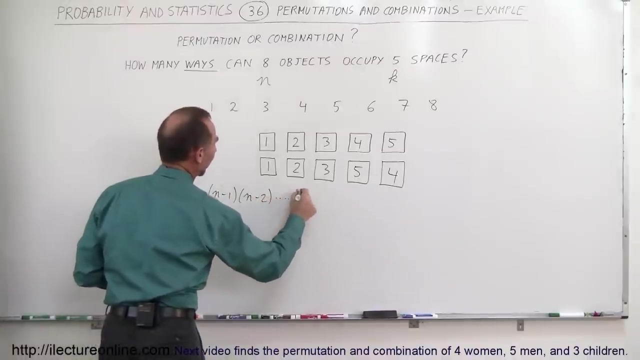 permutations is as follows: that the number of permutations. so starting with n quantities or n objects and k spaces, so this will be equal to n times n minus one, times n minus two, all the way down to n minus k plus one. So in our example, since there's eight objects and five spaces, n is 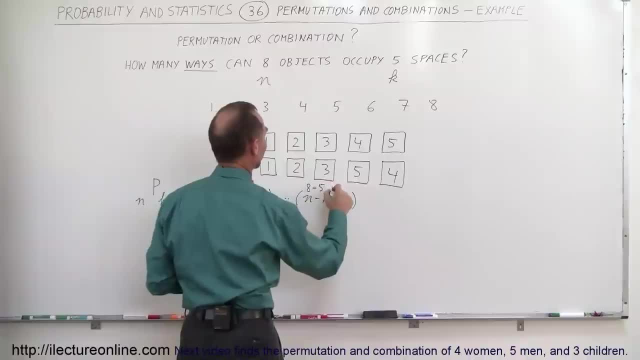 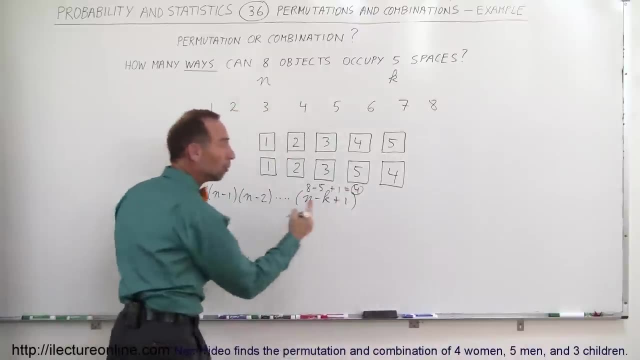 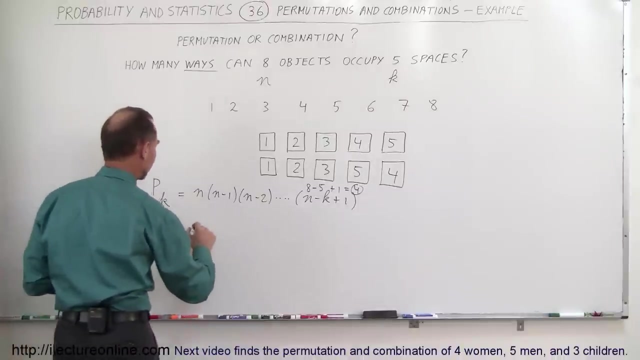 eight. k is five, so this would be eight minus five plus one. that would be three plus one, which is equal to four. So we go down from eight down to four, multiplying the numbers together, which means that the number of permutations with eight objects and five spaces is equal to eight times seven. 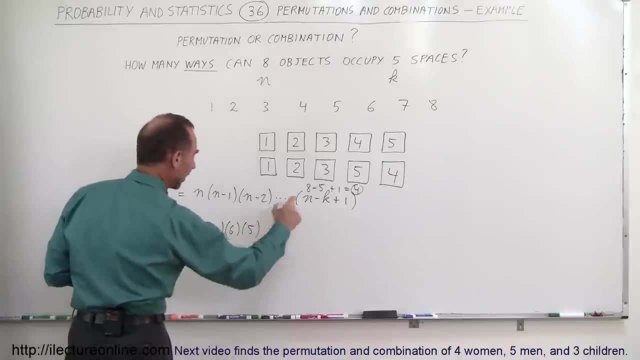 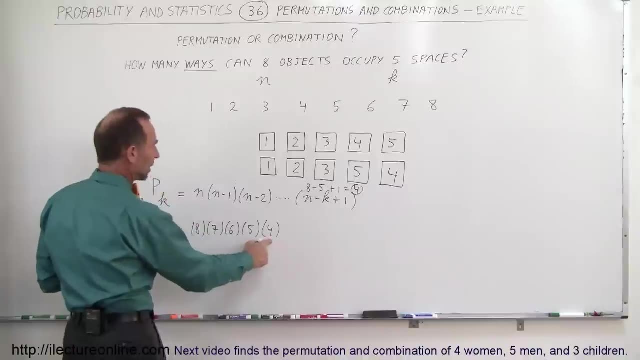 times six, times five and times four, all the way down to this quantity right there. Now we have to multiply these together. so five times four, all the way down to this quantity right there. So five times four is 20, times six is 120, times seven would be 840, so now we end up with eight. 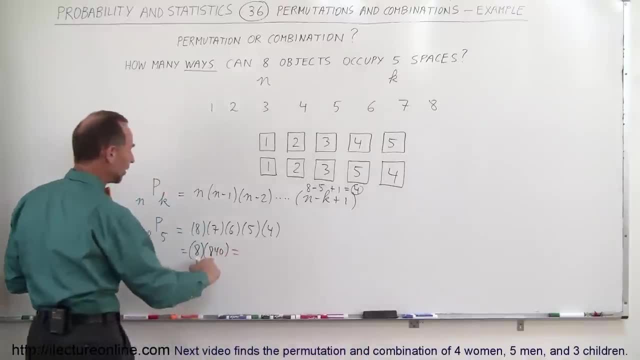 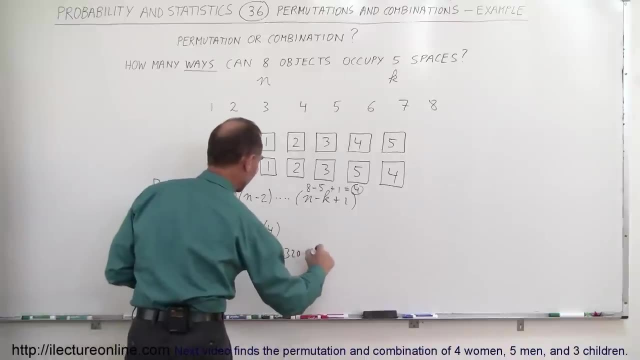 times 840.. Eight times eight is 64,, that's 6400,. plus eight times four is 32,, which is zero, that's 320, so this ends up being 6,720 different permutations. That's a huge number Just with. 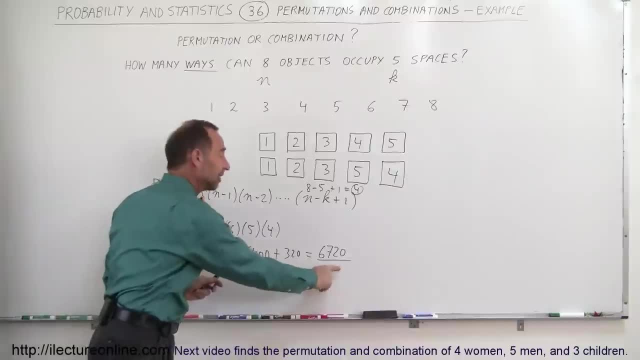 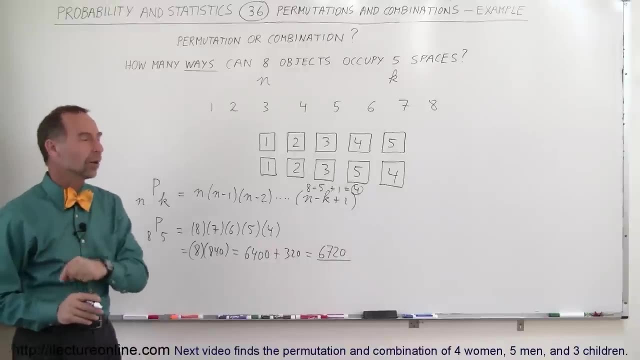 eight numbers and five spaces. you can rearrange them in 6,720 different ways. If it were to come to combinations, the number would be much, much smaller. Matter of fact, why don't we do that? What would it be if we just wanted to know the number of combinations? Well there, the equation. 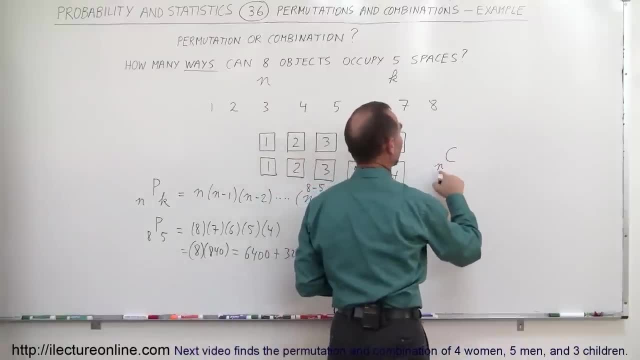 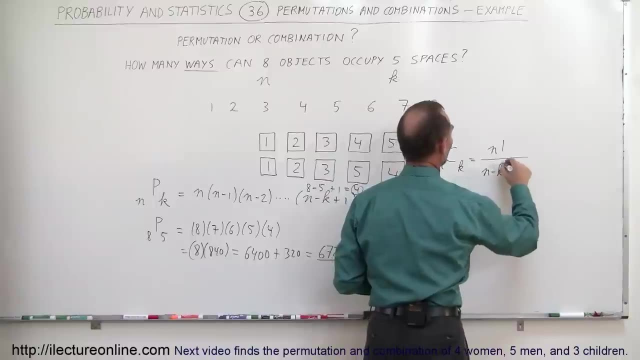 is as follows: The number of combinations. if we have n numbers and we have k spaces, this is equal to n factorial divided by n minus k. quantity factorial times k factorial In the case where n is eight and k is five. let's see what we get. So this is equal to eight factorial divided by: 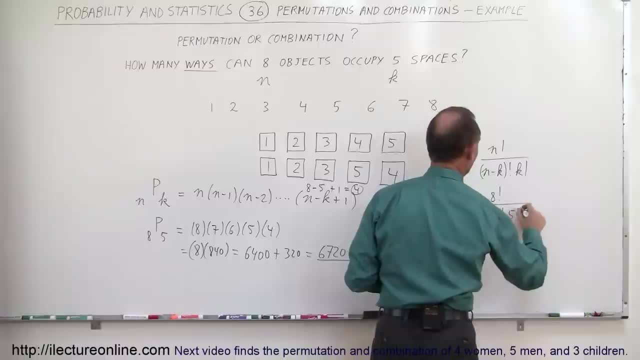 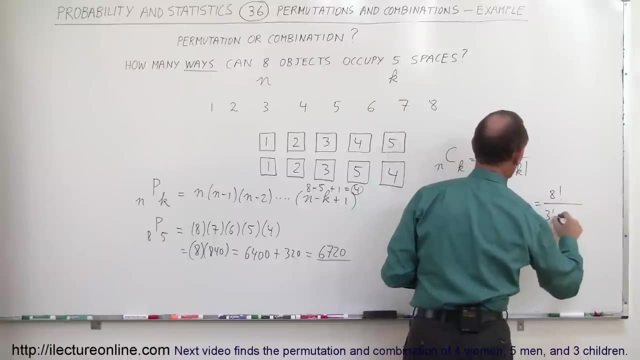 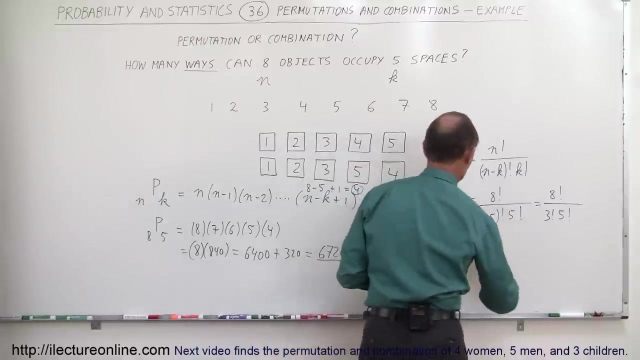 k, Let's just write out 8 minus 5 factorial times 5 factorial. Now again, simplifying this some more, this would be equal to 8 factorial divided by 3 factorial times 5 factorial. Now, remember that factorial means, for example, and I'll just write it out here: 8 factorial would simply be 8 times. 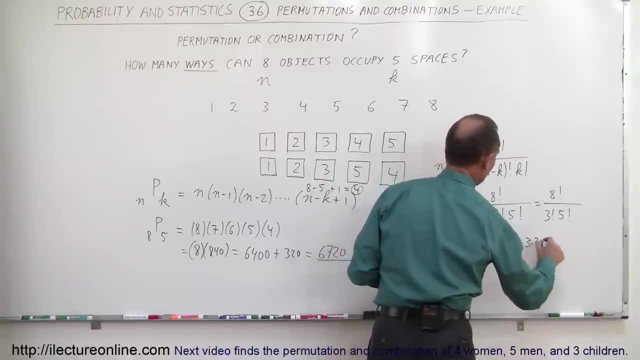 7 times 6 times 5 times 4 times 3 times 2 times 1.. Divide the whole thing by 3 times 2 times 1 and multiply that times 5 times 4 times 3 times 4 times 5 times 4 times 3 times 4 times 5 times 5 times. 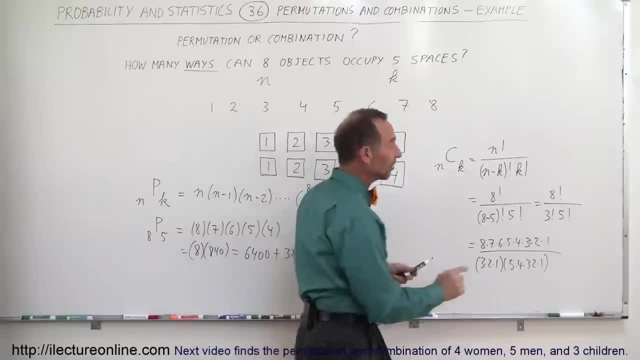 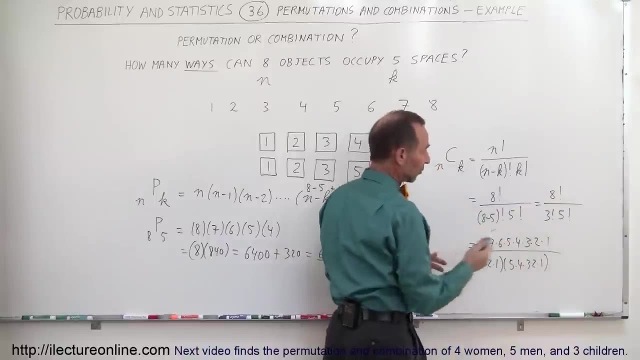 3 times 2 times 1.. Usually what we do is we realize that 5 factorial will cancel out with the bottom five numbers of 8 factorial, which only would leave 8,, 7, and 6,, which is indeed what. 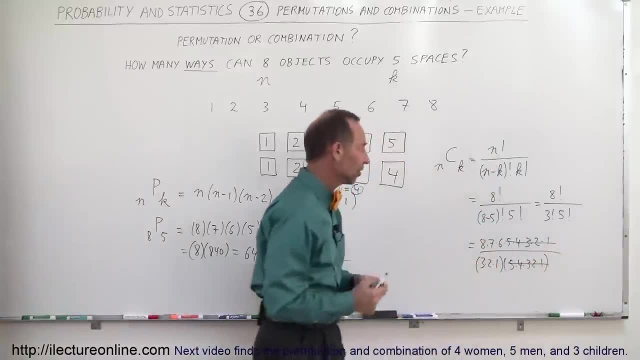 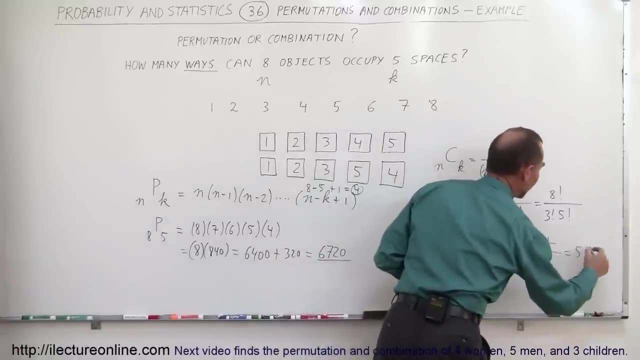 happens when you simplify: cancel these out, so you end up with 8,, 7, 6 in the numerator, 3, 2, 1 in the denominator. Then notice this: 6 cancels out with this 6, and you're left with 56.. So if the 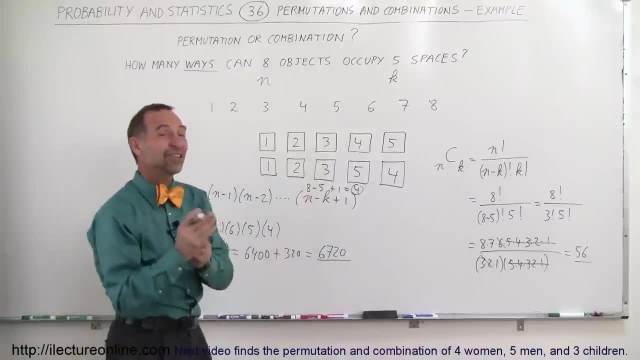 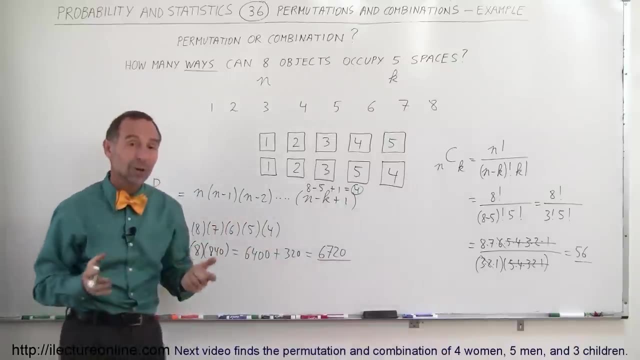 order doesn't matter. realize then that you only have 56 combinations. If the order does matter, you have 6,720 permutations, and that's how you know the difference between permutations and combinations, and that's how we do it. 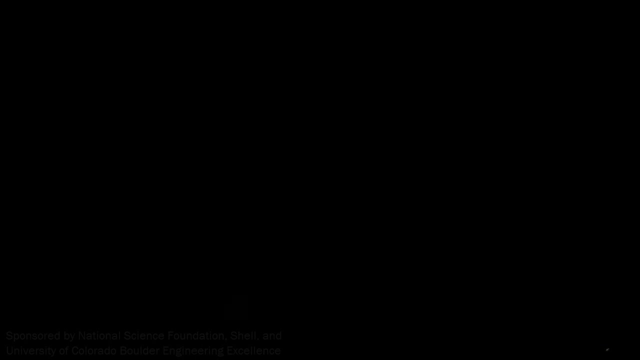 In this screencast we will discuss the concept of cascade control, how it's implemented, and discuss the block diagram for cascade control. So before we do this, we have to think about why we would want cascade control The majority of all processes that are being